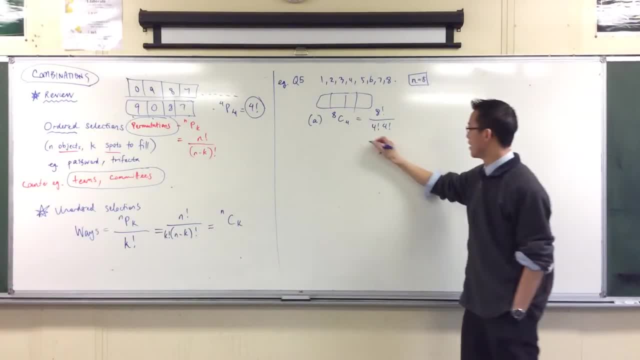 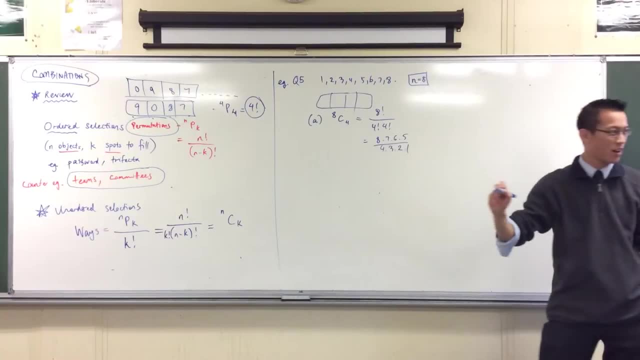 That's four factorial, four factorial done okay. So let's see I'm going to get eight by seven by six by five On four by three by two by one. Is that okay? One of my four factorials cancelled. 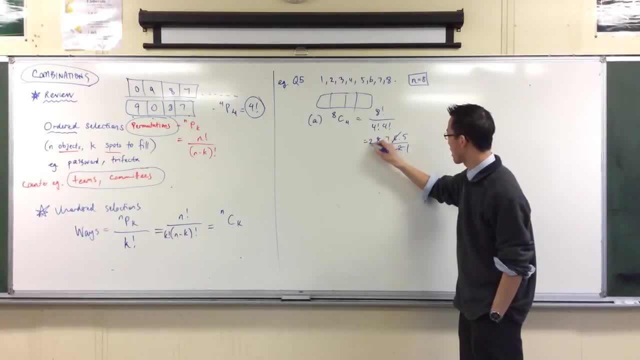 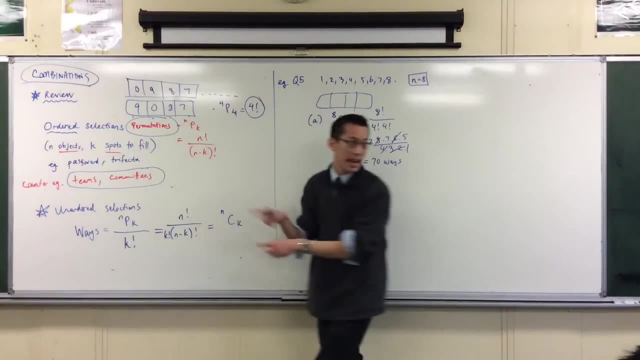 I can cancel that. I can cancel that. That looks to me like seventy. Yeah, It's okay. I don't expect you to do that. However, just as a helpful note, it's really good to have these in the back of your mind as you do them. 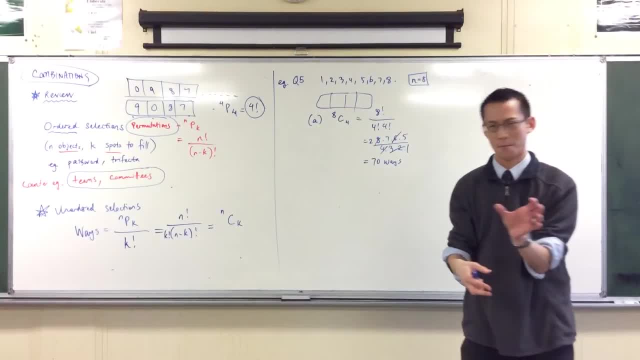 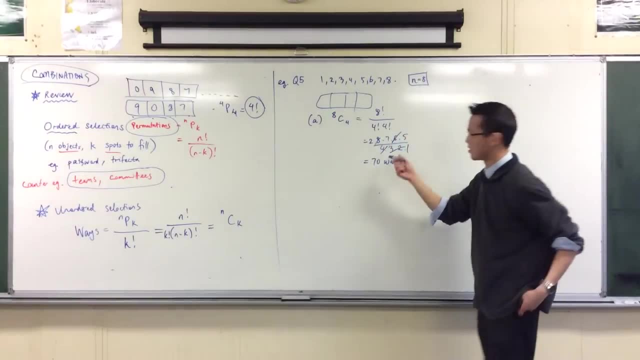 And don't just rely on your calculator to work those out. when you're doing identities and all that, It's really helpful to be able to just go. I know exactly what that stands for And this is the way that I practice. So seventy ways, no problem. 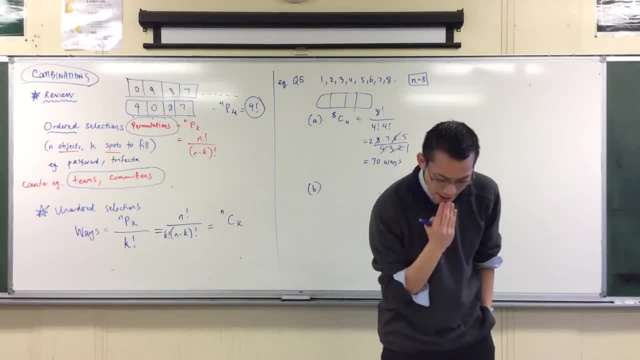 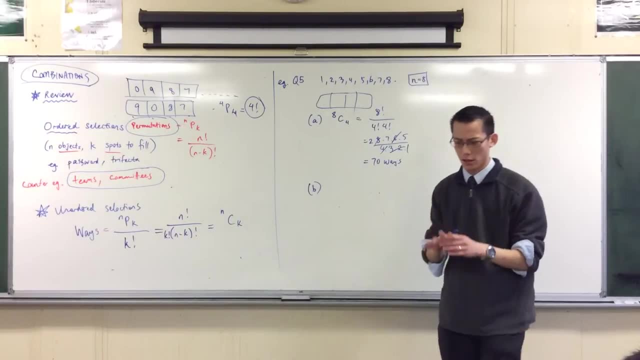 Let's start to add some conditions in. There are two odd numbers and two even numbers, So now I have to restrict a little bit. Let's think about it one step at a time. First, I want to pick a pair of odd numbers. 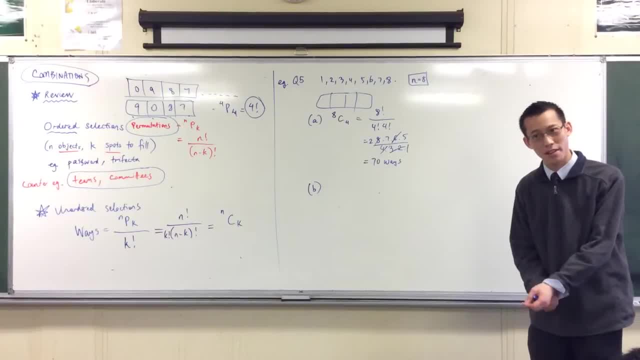 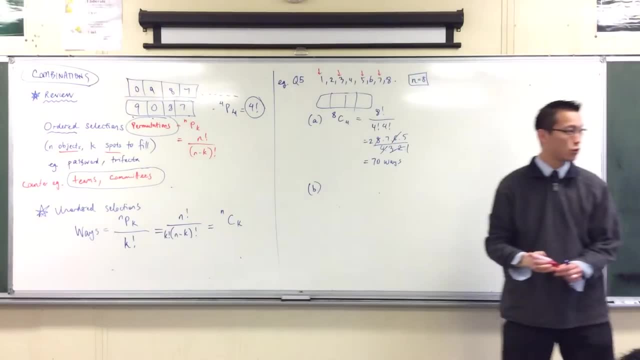 So you have a look at your sample space and you think how many odd numbers are there, And the answer is there are four. One, two, three, four. Cool, So now, instead of n being eight, right For this situation, I'm just picking from odd numbers, right? 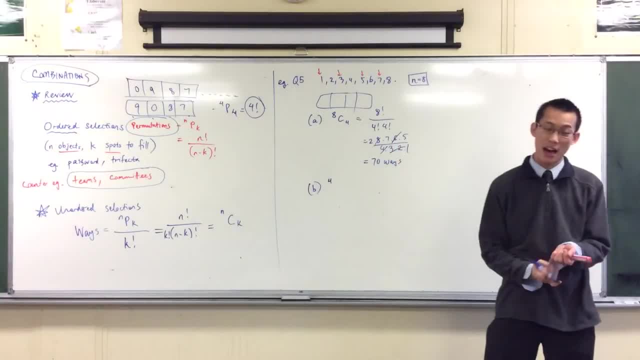 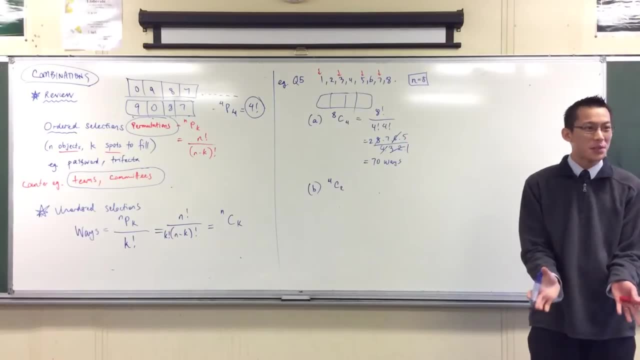 I only get to choose from four right Now. how many do I want to pick? I want to pick two of them. Okay, great. So now I've picked out those two, What do I do with the others? I look at my even numbers and I repeat the process. right? 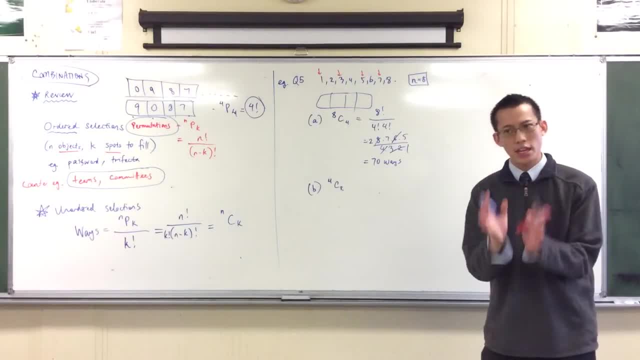 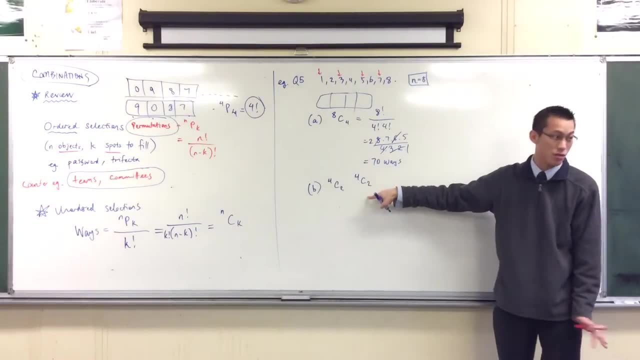 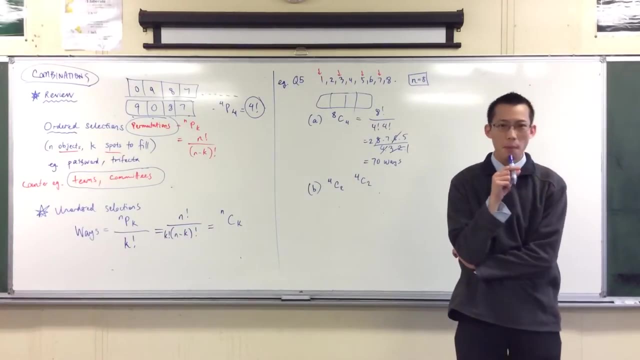 Now pause for a second. We're thinking about this under the context of probability, right? So I know that for the evens there's going to be four, and then I have to choose two of them again. But in between, here, am I adding or am I multiplying? 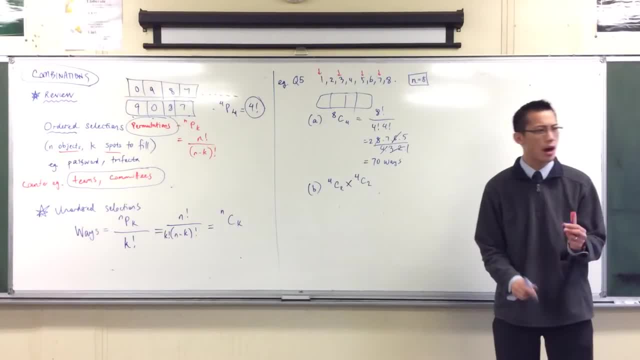 And the answer is: I am multiplying, I'm not adding. But the question is why? Because how will you be able to tell when it's a bit tricky right? How do you know that it is multiplication and not addition? When do we use addition and when do we use multiplication? 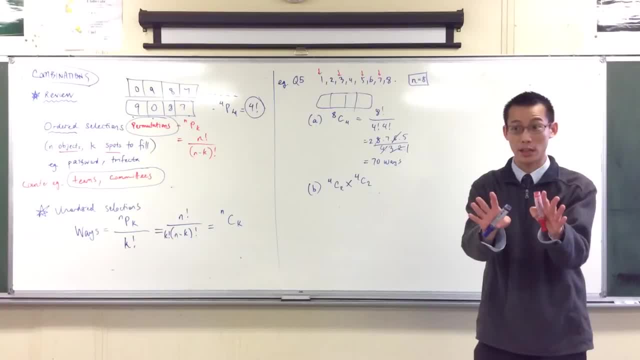 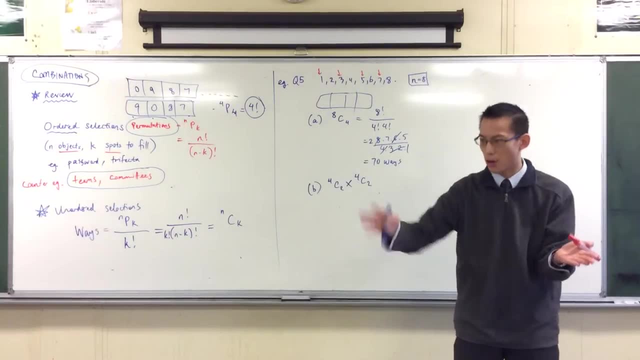 When did the product rule and addition rule come in in terms of probability? Yeah, you can either think in terms of independent and dependent events, or the way that I've catched it in class has been either simultaneous events or not simultaneous events. okay, 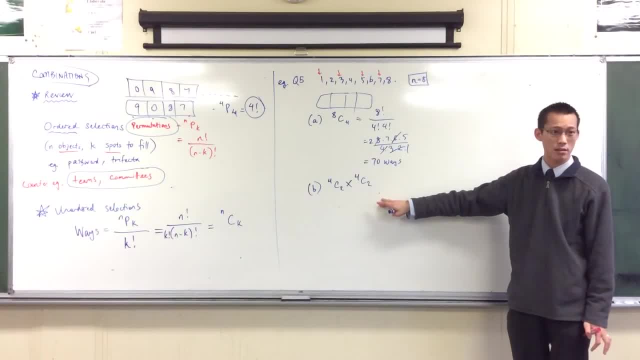 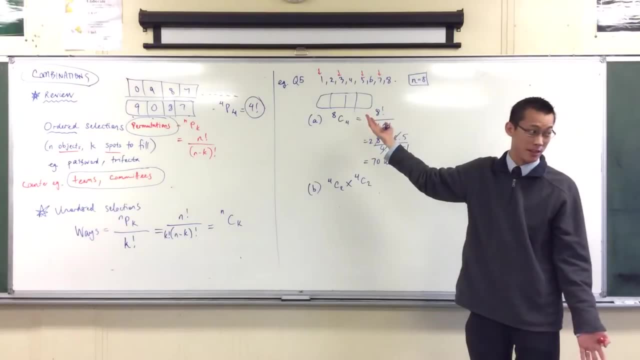 Now here's the thing: You want to end up with four numbers at the end, right? So you need these two and these two at the same time. If you don't have all four, then you don't have the four numbers that you were meant to come up with. 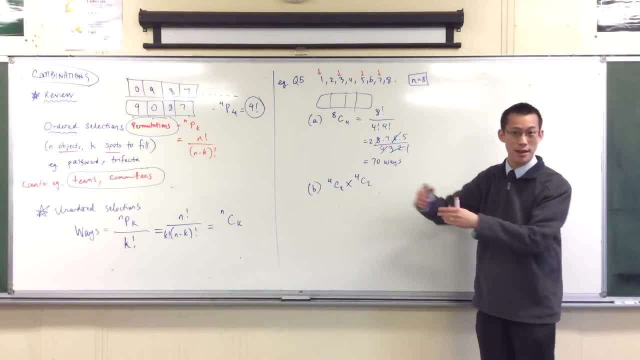 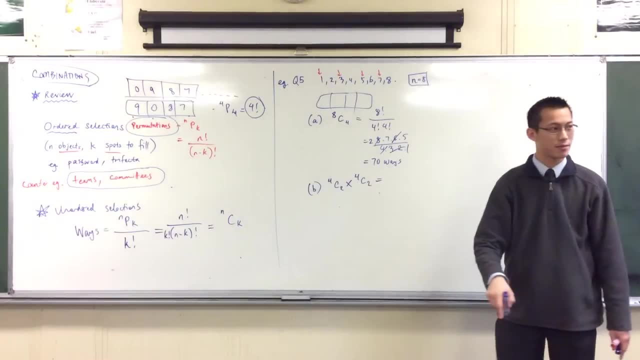 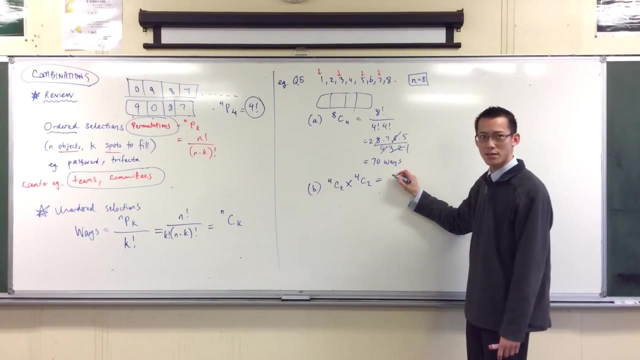 So, being that you have to have them at the same time. that's why I multiply. okay, All right, Let's see Four choose two. So we're going to have to reach for a calculator on this one. I think this is four times three. on two times one, because one of my two factorials is cancelled. 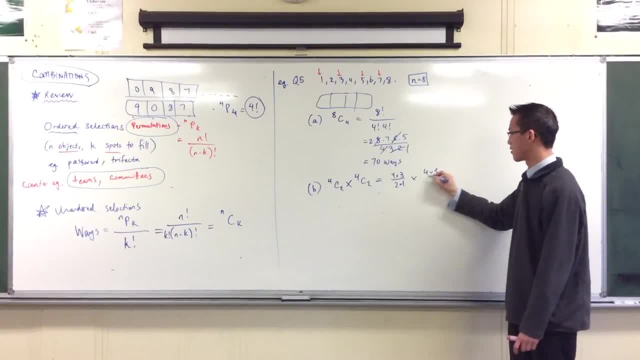 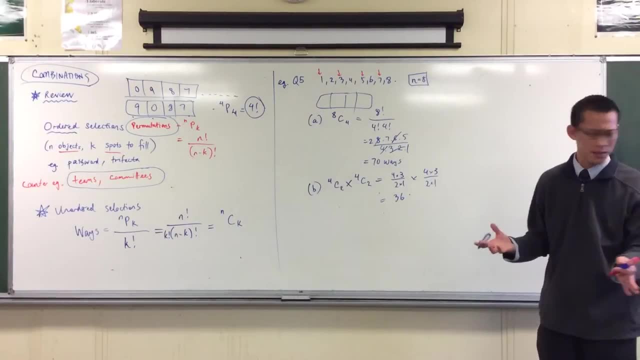 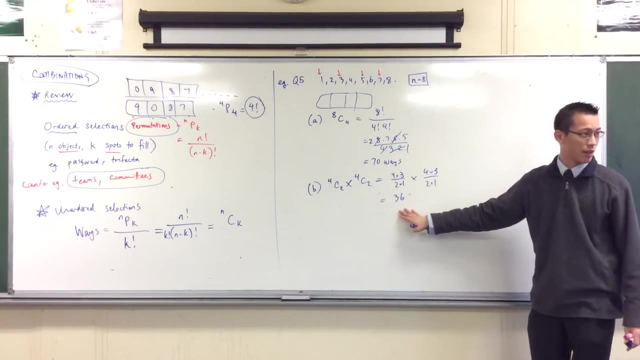 I'm going straight to this line, So that's six. and then you're doing it again, So that's 36.. 36 ways, That makes sense. There should be far less ways to do it than this. This is our big sort of sample space, if you like, and now I'm restricting, okay. 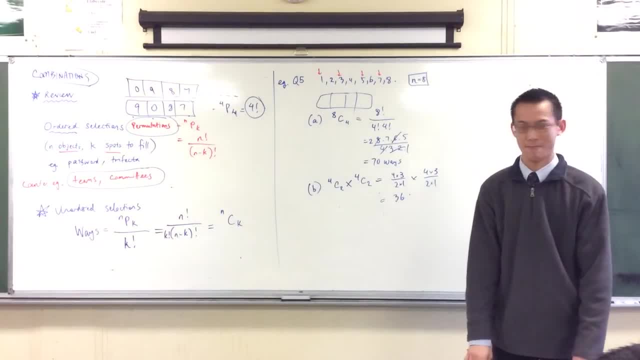 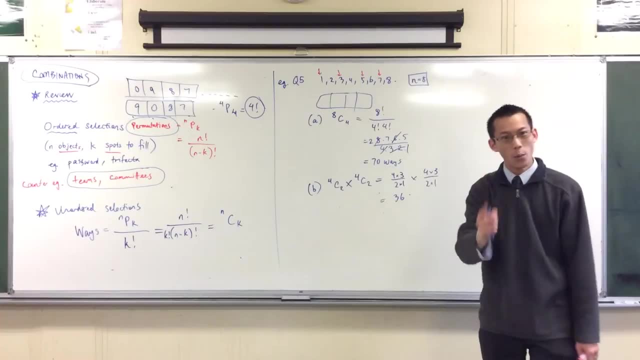 So, by the way, let's just quickly turn this into a probability question. all right, This is not that hard. Suppose four numbers out of these are picked at random, What would be the probability that two are odd and two are even? 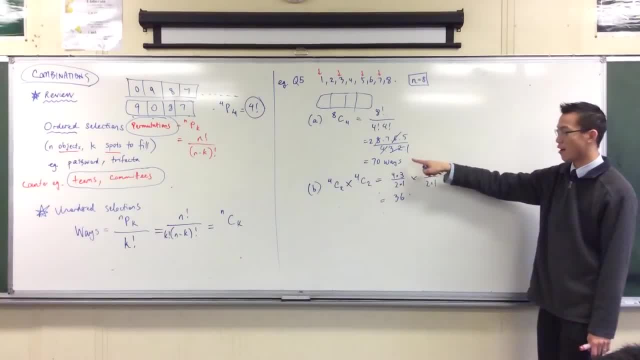 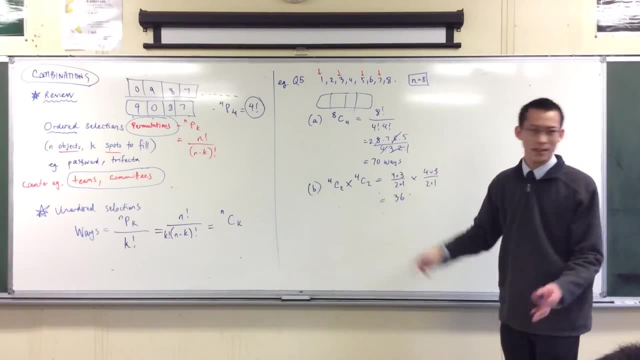 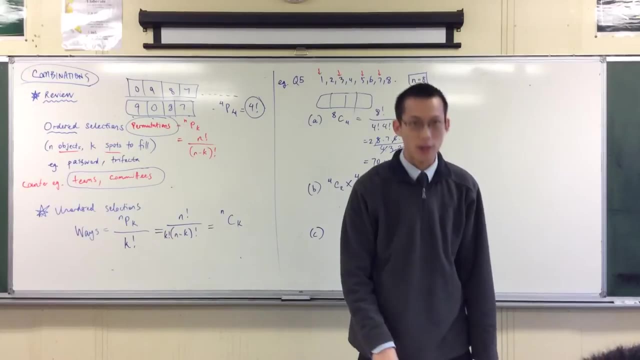 And the answer is: look favorable outcomes over sample space. So it would be 36 on 70.. Does that make sense? Do you see how they're going to use this in the future? Let's add another condition. There is exactly one odd number. 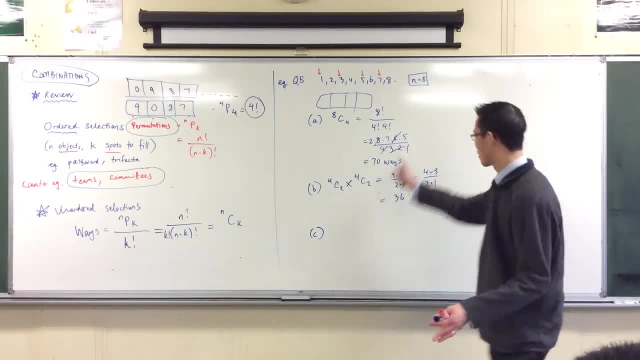 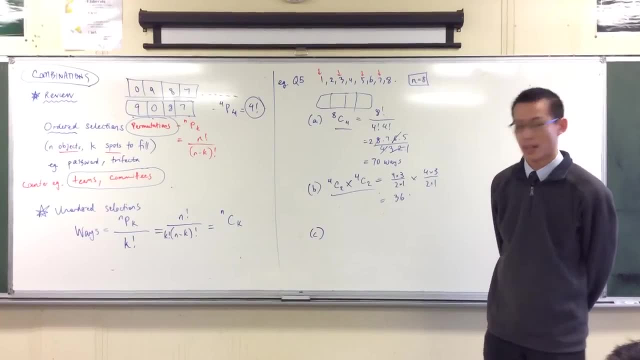 Exactly one odd number. Okay, I've walked you through these ones and the ways that I set them up. How would you like to suggest I set up this one? Okay, So hold on. I heard 4C1 over here. 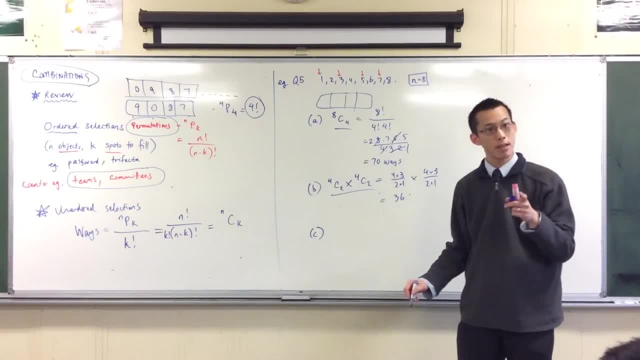 Why? Why 4C1?? Because you can only have one odd number. Okay, So I've got four odd numbers to choose from right, But I only want one of them. I don't want a pair, I don't want it just free for all. 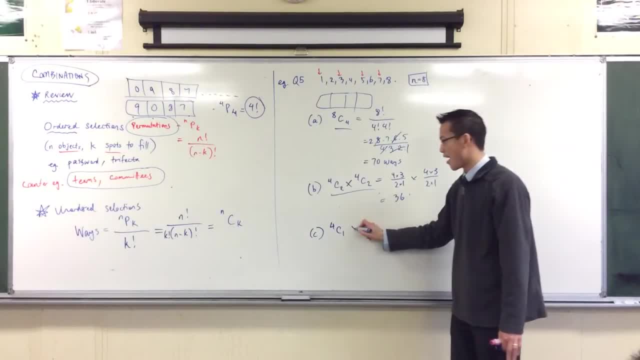 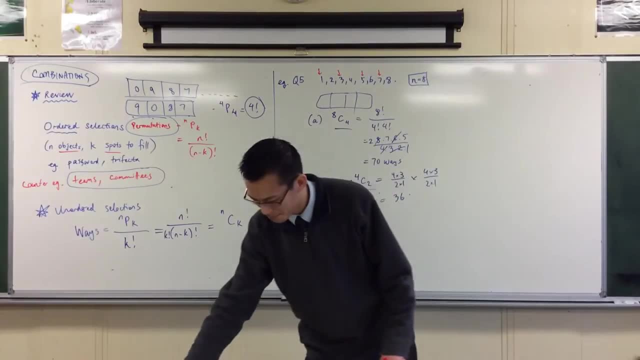 Okay, I've got to pick just one, And then, of course, you've got the other, even numbers- but you've got to choose three of them to make up your four, Okay, So I don't know what that is, but I wrote it down. 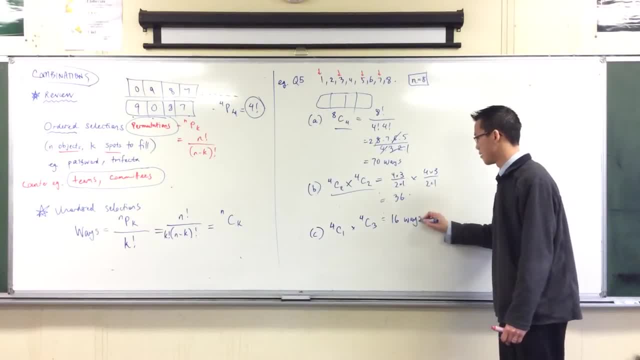 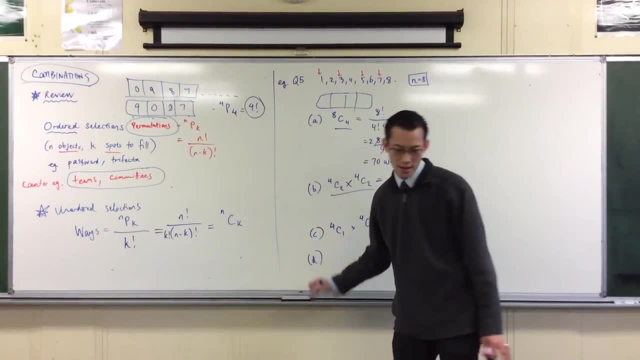 I think you end up with 16 ways. All right, Okay, That's not so hard. We're starting to get the hang of it. D: this is the. It's not the last one. All the numbers must be even. 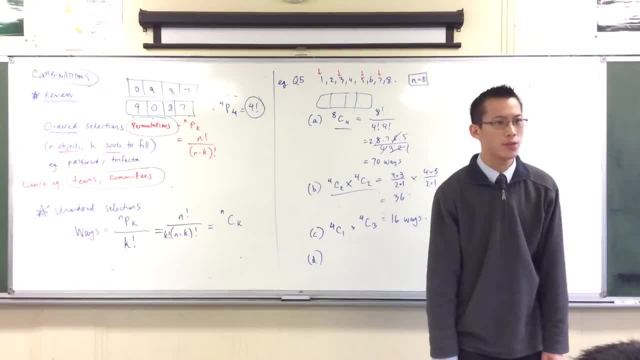 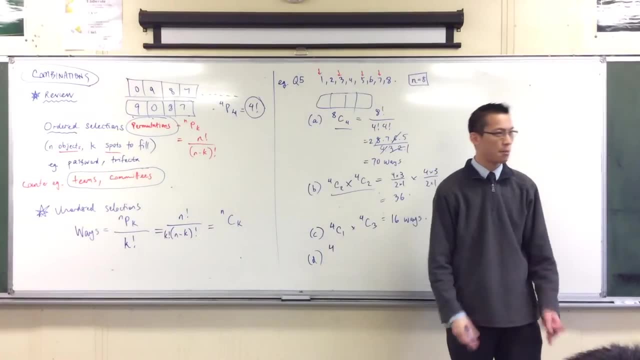 All the numbers must be even. So what have you done? What have you done? You still have to pick four, but then you've just kicked out all of these options, Right? So now you only have four to choose from, but you've got to pick all four. 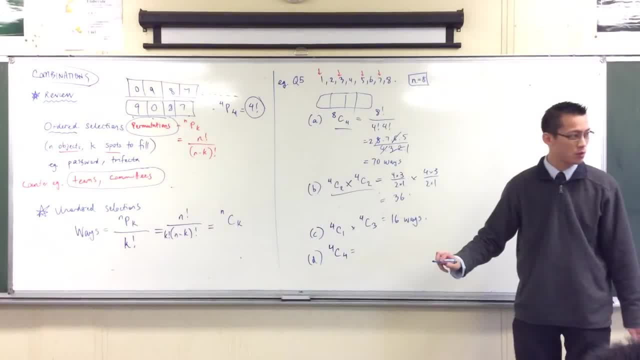 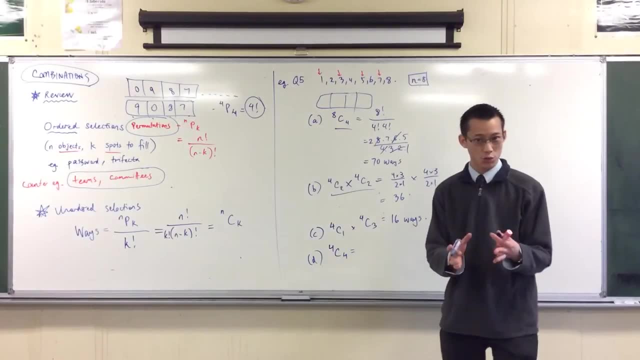 Right. So choose four, Right, Or choose four, That's all right. So what's that going to be Now? let's just go back to our factorial notation. Right, This is going to be four factorial on four factorial, nought factorial. 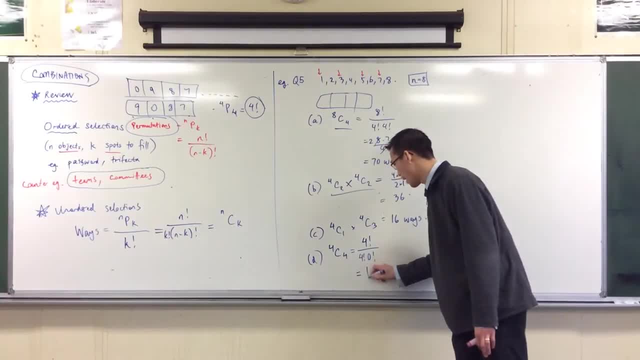 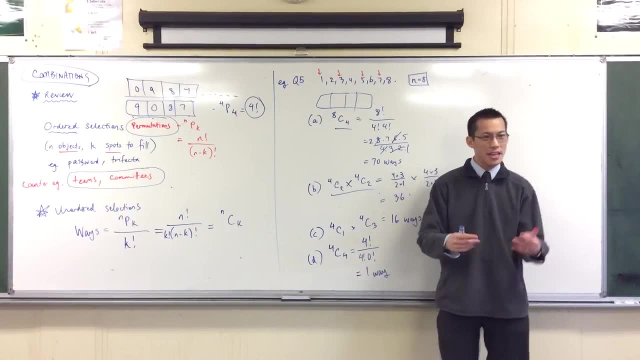 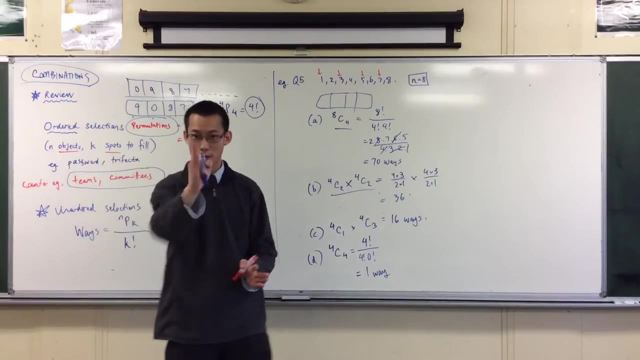 Nought. factorial is one Hold on, It's just one way. Why is that? Because you've picked all four Right Now. think back to me over here with my password, Right? I'm like: look, if I do 4P4, there's four to put in the first spot, three and then two. 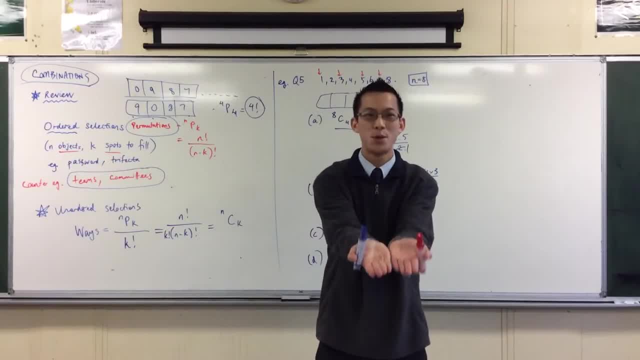 and then one Right. So I'm going to pick four factorial And I hand over my four factorial different options to you, Right, And then you come to this situation. You're like they're all the same, You know. 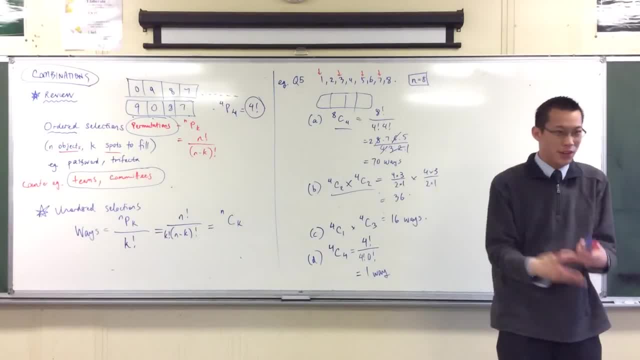 There's 2,, 4,, 6,, 8.. And there's 8,, 6,, 4,, 2.. You've given me the same set of four even numbers. There's only one way, really, that you've given me. 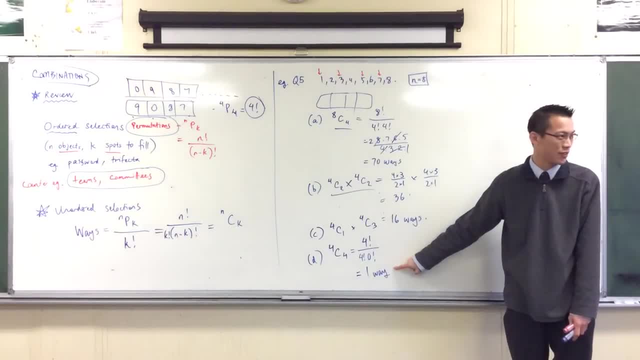 Okay, Does that make sense? So you're trying to transition between the different noughts. Last one: Read it carefully: There is at least one odd number. So this is similar to the exactly one odd number, But there is at least one odd number. 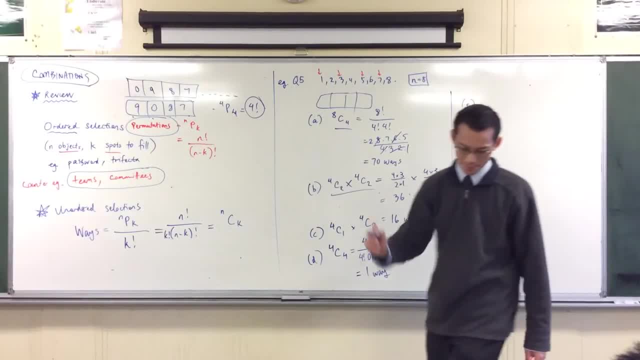 So this is similar to the exactly one odd number, But there is at least one odd number. So this is similar to the exactly one odd number, But there is at least one odd number. Read it carefully: There is at least one odd number. 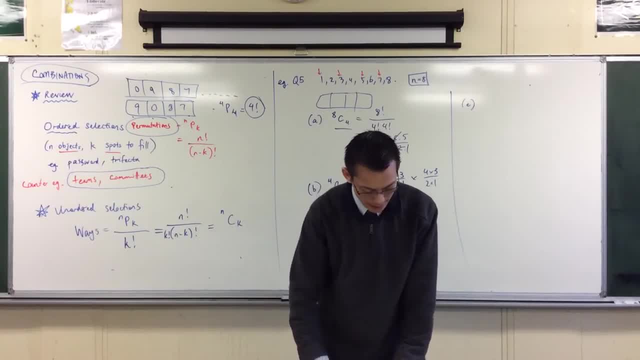 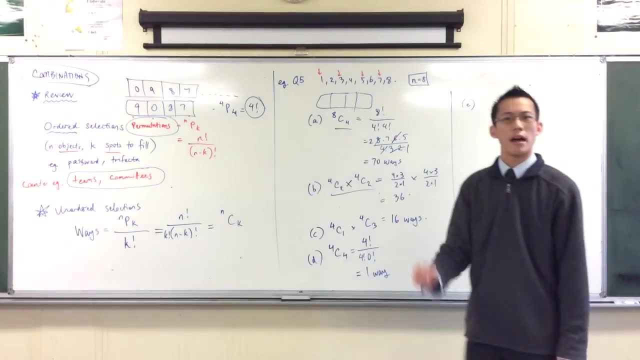 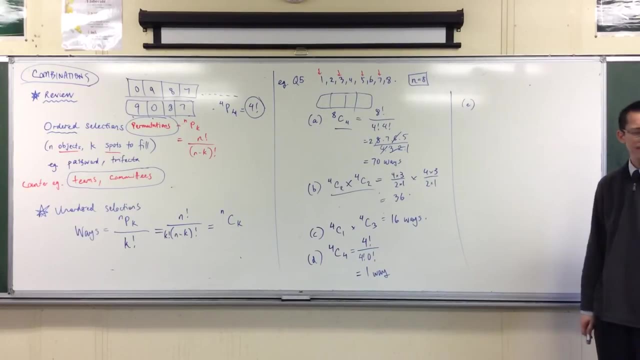 So this is similar to the exactly one odd number, But you can have one odd number, or you can have two odd numbers, or three odd numbers or four odd numbers. Okay, So how should we approach this? Any suggestions, Any 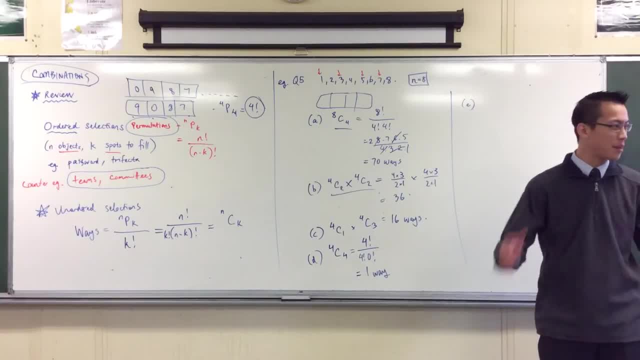 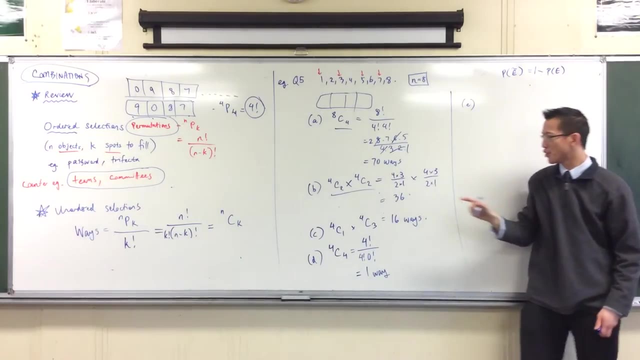 Does anyone know? Okay, Okay, I'm hearing someone say: a complement, Now hold on. the idea of a complement makes sense in probability because it's like, okay, if you've got the probability of the complement right, it's 1 minus the probability of the actual event, right, But you don't do 1 minus here, right? So what do you do? 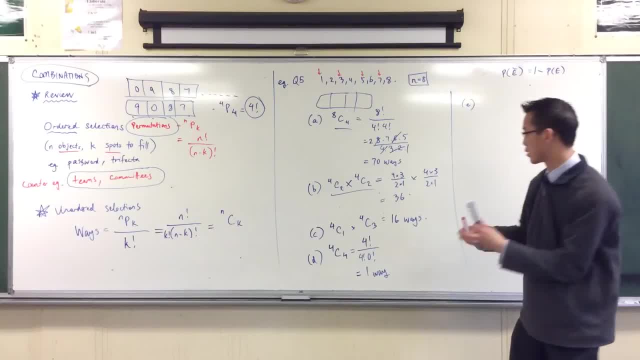 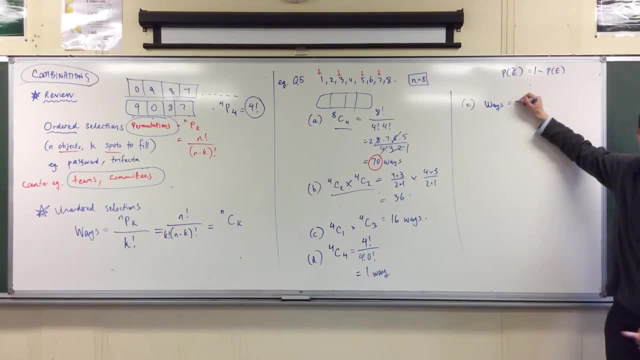 Okay. so you think of the whole sample space which we already worked out. It's this guy, okay. So therefore, the number of ways will be okay, it's going to be 70, that's my whole lot minus. now, what is the opposite of the event they're asking for? 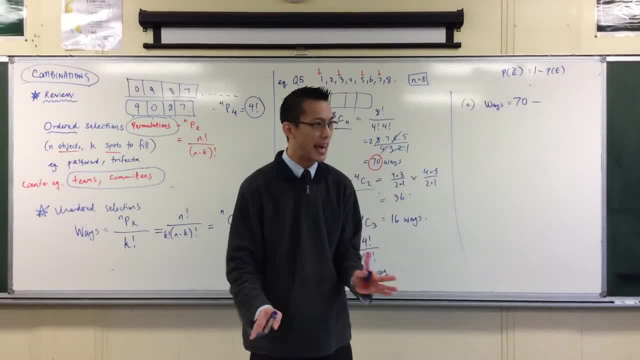 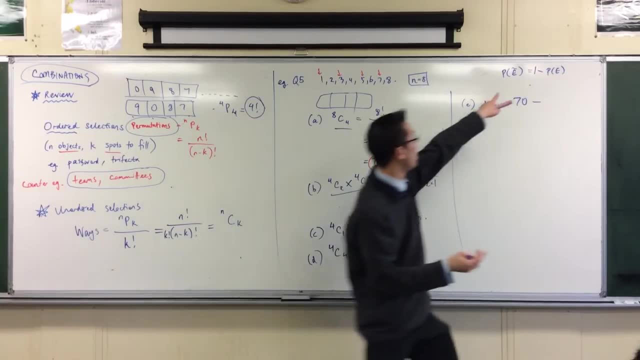 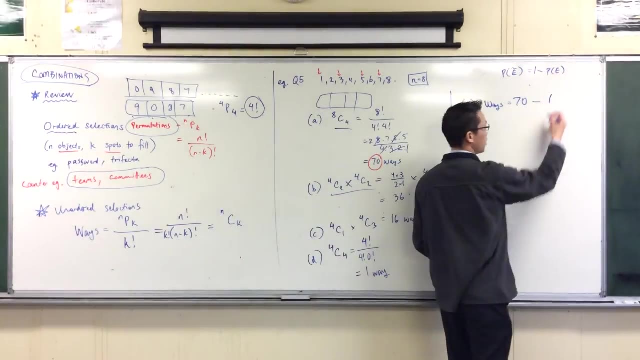 At least one odd number. The only way to not get at least one odd number is to get zero odd numbers. That's the only way to get to be the complement right, And we just worked that out. That's getting all the even numbers right. So it's 70 minus 1.. That's the only way. okay, So you get 60.. 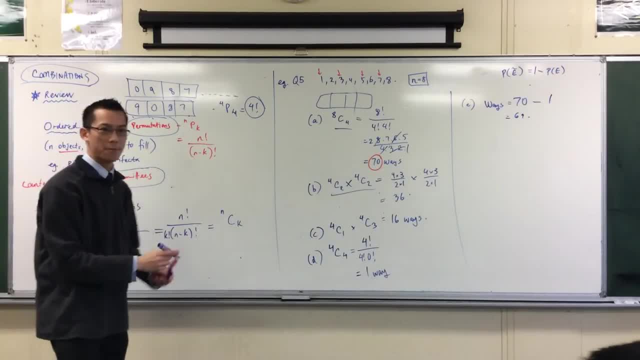 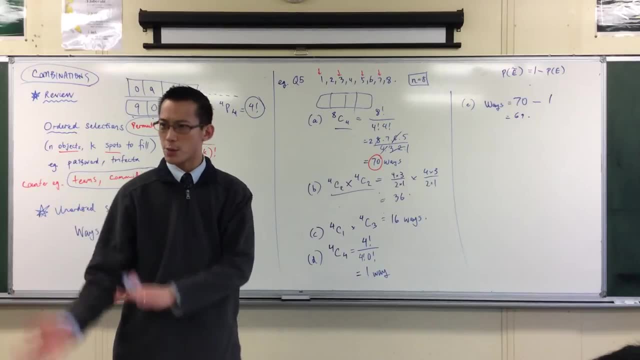 And, by the way, just for the sake of it, right, that was the smart way You guys have gotten your head into the space, which is really good. okay, What would be? because it's not the only way. with these probability and arrangements questions, there's almost always multiple ways to do it. 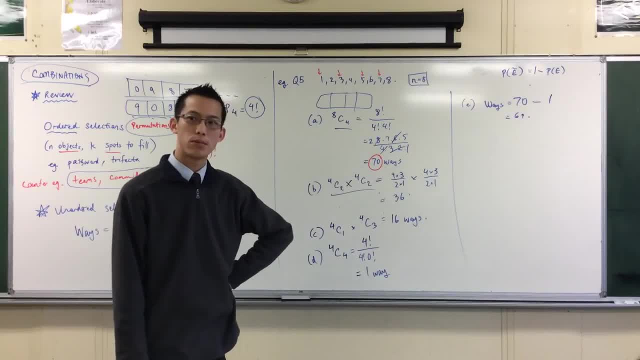 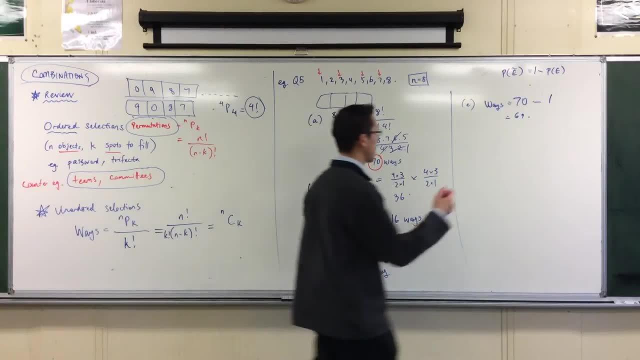 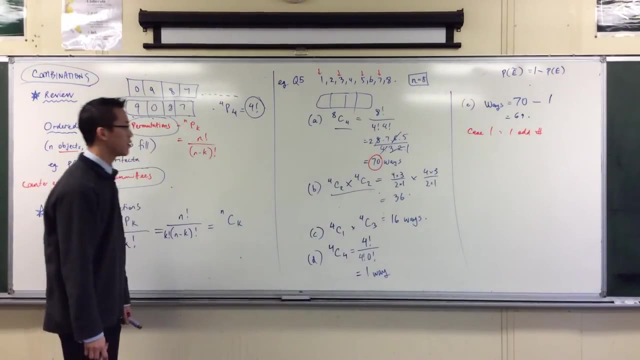 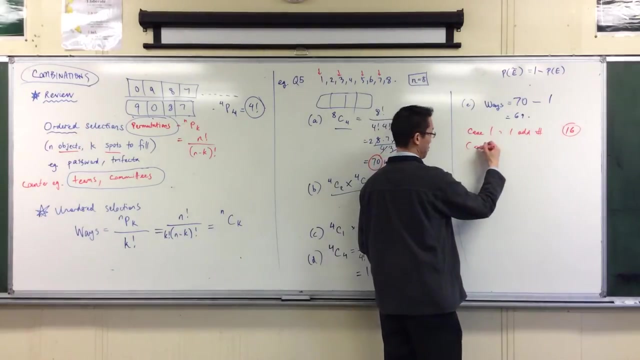 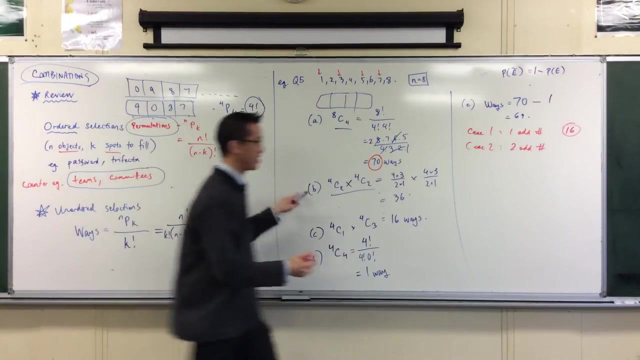 Even though it might not be ideal. what would be another way to approach this? You think of different cases, and there are four of them. okay, You can go. case one: One odd number. right, One odd number. We've done that, haven't we? Where is that? That's this one, right, 16.. Okay, What would be case two? Two odd numbers Now hold on. Haven't we done that one? That's here, isn't it 36. Okay? 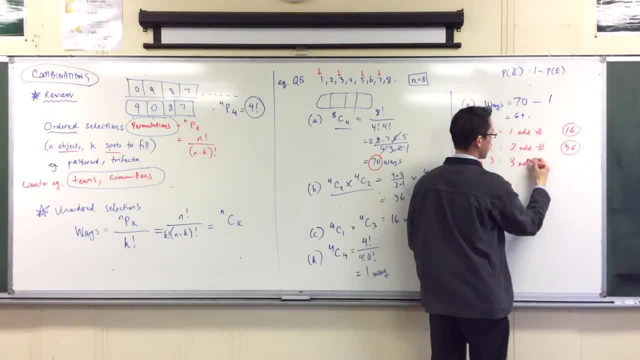 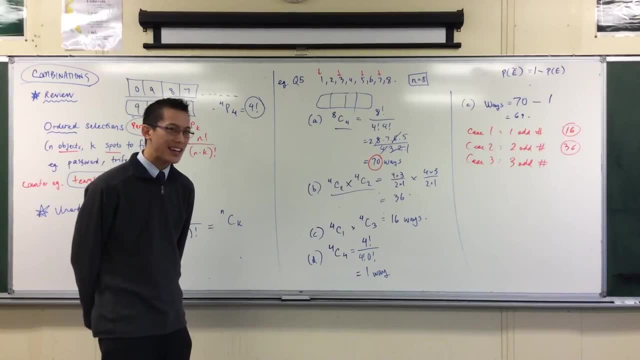 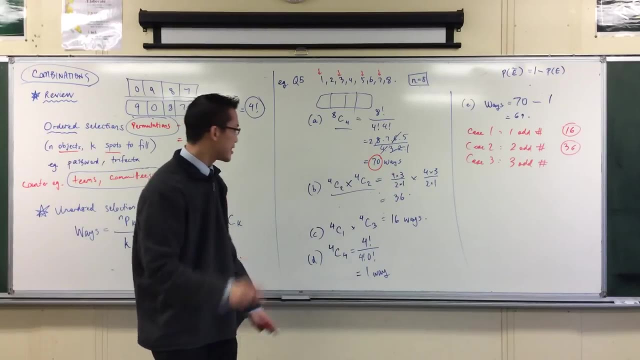 Case three: Now, this is interesting: Three odd numbers. okay, We haven't done this one, but we kind of have Think about why. okay, None of these questions said what about three odd numbers, But they did say what about three even numbers, And that's exactly the same right. 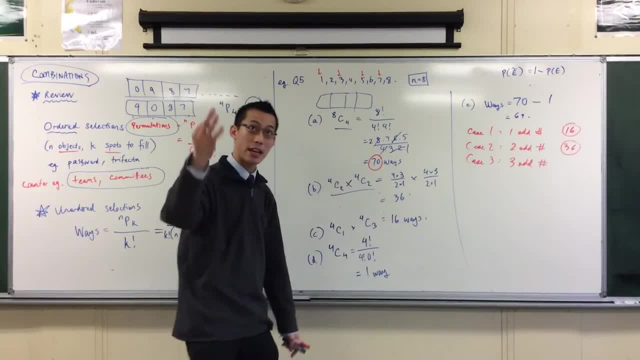 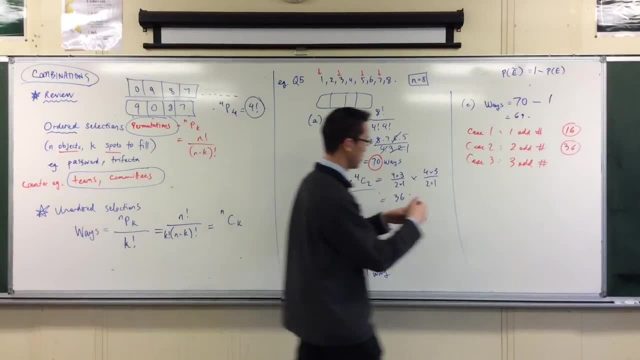 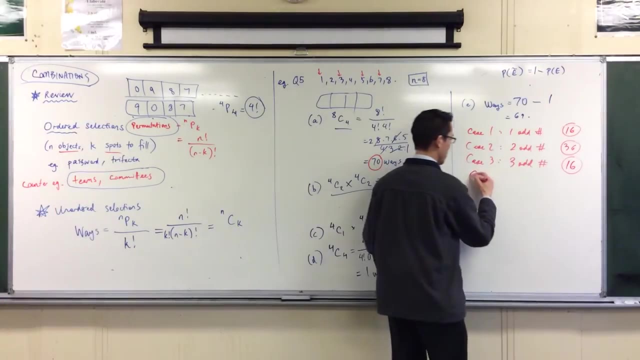 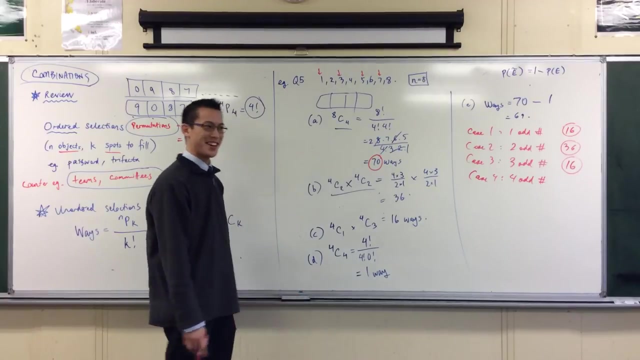 Because there's the same number of even numbers and odd numbers, right, Picking three evens. there's going to be the same number of ways to do that as picking evens, Picking three odds, right. So this is also going to be 16.. Yep, There's the last case, right: Four odd numbers, which, again, we have not worked out, but we've worked out one close enough, namely four even numbers. same scenario. 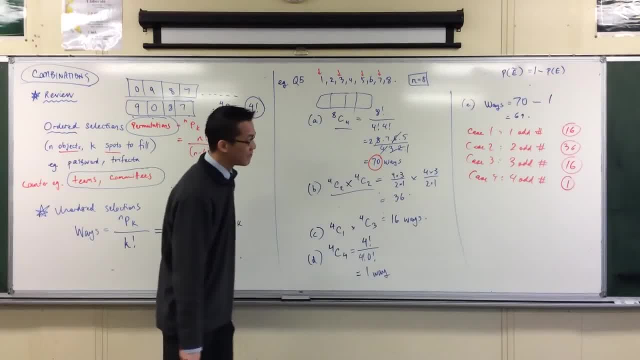 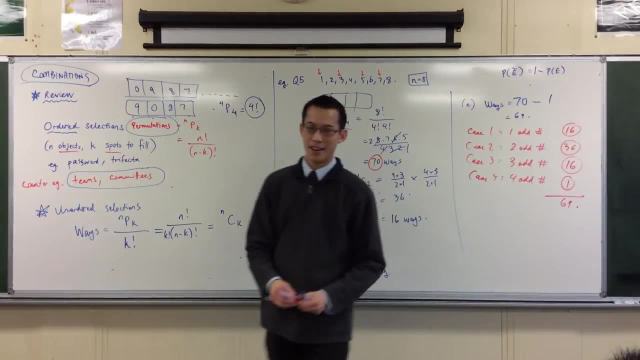 So this should be in one way okay, And it looks to me. I mean, my number computing is not that good in this time of morning, but it looks to me like that. Okay, Of course you can see the complement When I write it out like this. you can see the complement almost sort of by its absence, right? 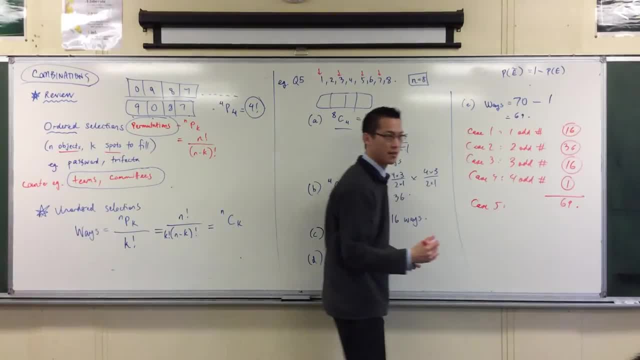 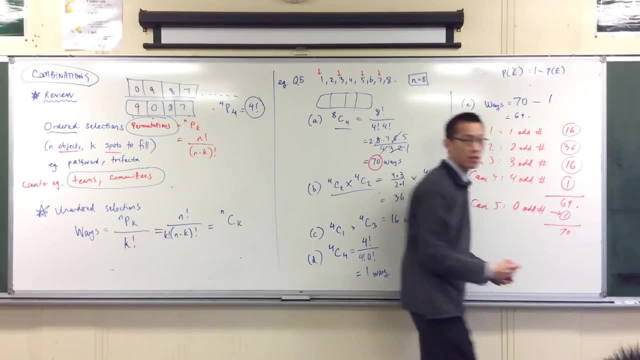 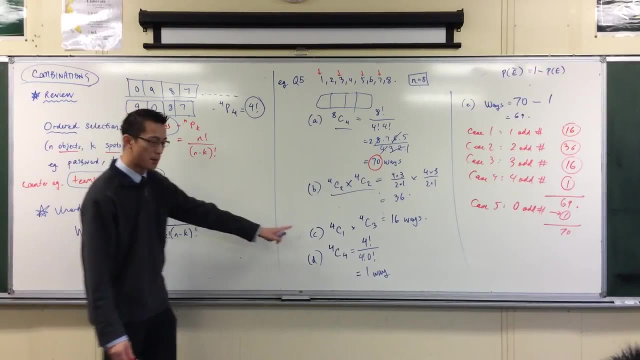 What's case five The case you're not interested in: No odd numbers, right? Zero odd numbers, which, of course, is the complement that you worked out before. That's the one which gives you 70 in total, your sample space. So there you go, Simple situation. Let me just quickly formalize this complement idea for you, right? 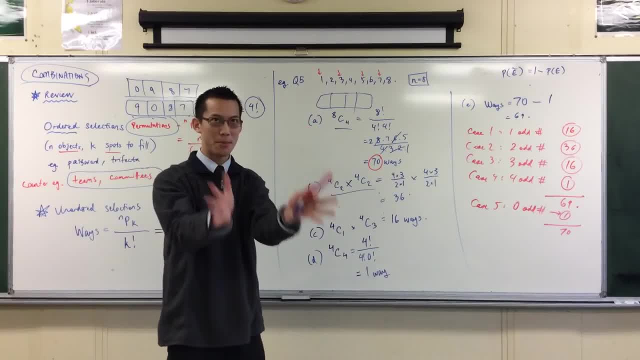 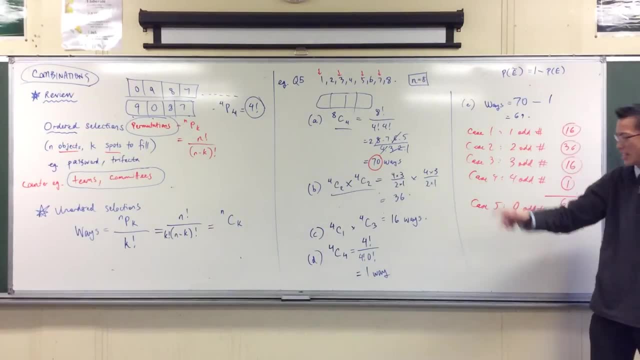 Remember we said picking three Three odd numbers is the same as picking three even numbers, right? So, if you like, it's kind of like let's think about your team, right? So, if you want to choose five people, right. Sorry, you've got five people to choose from, right, And you want to pick four of them. 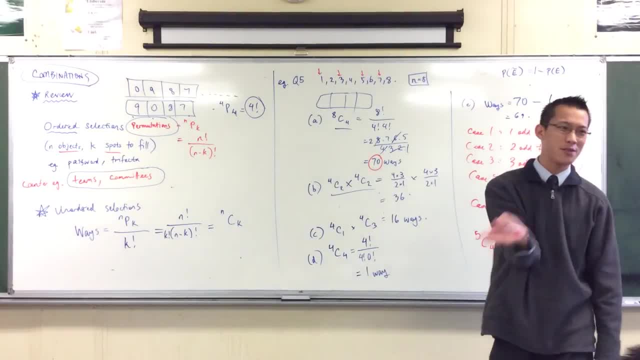 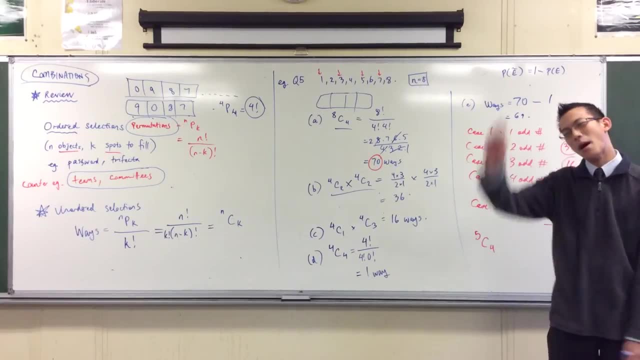 Well, you might as well just say like: can you imagine, are any of you like me, that person in the schoolyard where you know the captain from one team and the captain from the other picks out, picks out, and you're like, I'm always going to be last, okay. 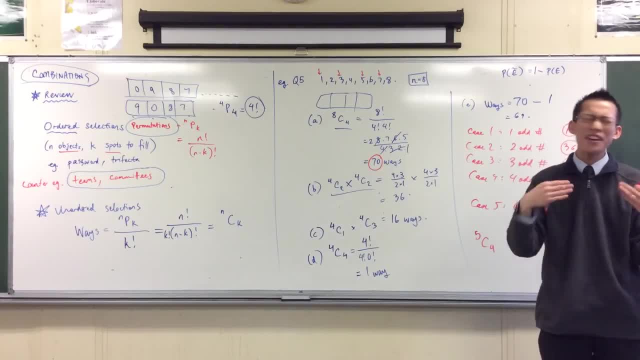 Okay, That's the least athletic prowess of the whole people here, right? Why don't you just pick me first and say: I don't want you on my team? That's the same thing, isn't it? That's the same.